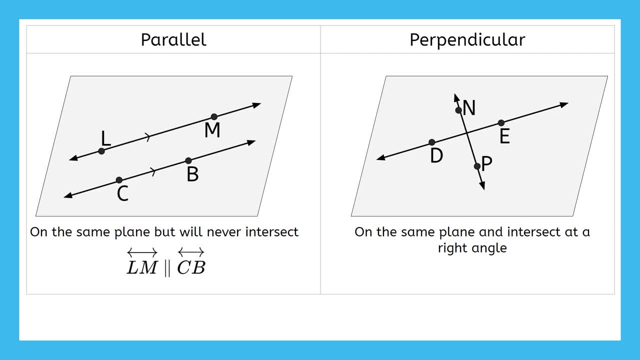 Specifically, they intersect at a right or 90-degree angle. In this example, lines NP and DE are perpendicular. This symbol is used for perpendicular when writing this out And this symbol is used for perpendicular on a drawing. It looks like we're putting a little square in one of the right angles. 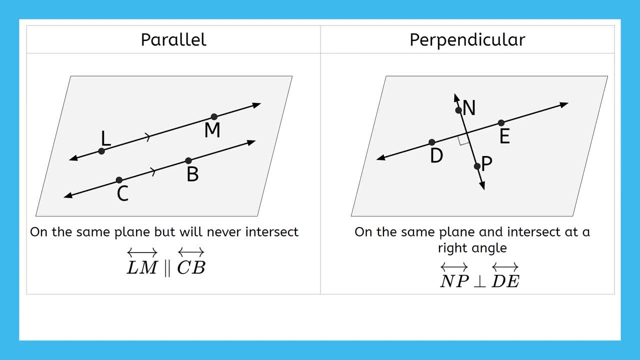 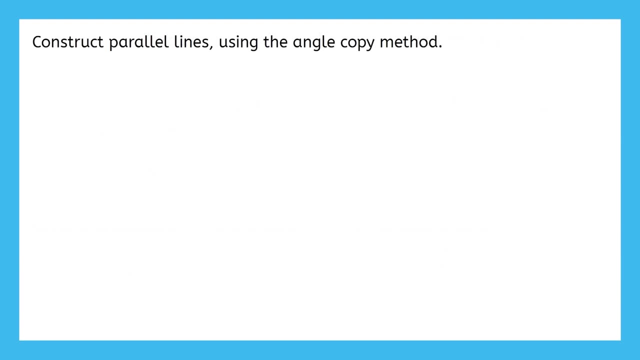 And since there are four right angles here, you could put this symbol in any of them. Pause the video here if you need more time to write your notes for this. Next up, we're going to start some constructions. We're going to learn one way to construct parallel lines together. 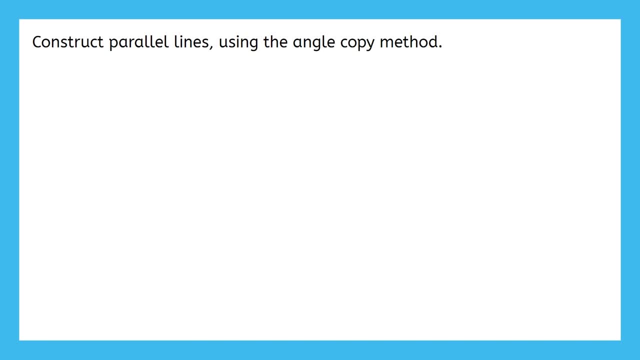 And then you'll have an opportunity to explore two more ways in your activity later on. The method we're using is the angle copy method. It'll be best to create this in your notes as we go, so remember to pause the video any time you need to catch up or rewatch something. 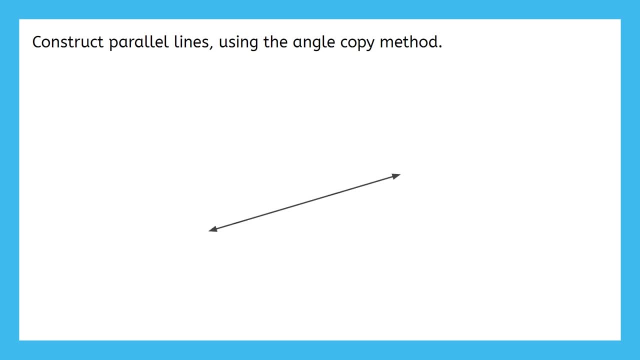 Start by drawing a line like this. Then use your straightedge to draw a segment going through that line that you can tell is definitely not perpendicular to the original line. Place a point on this new segment that you would like your parallel line to go through. 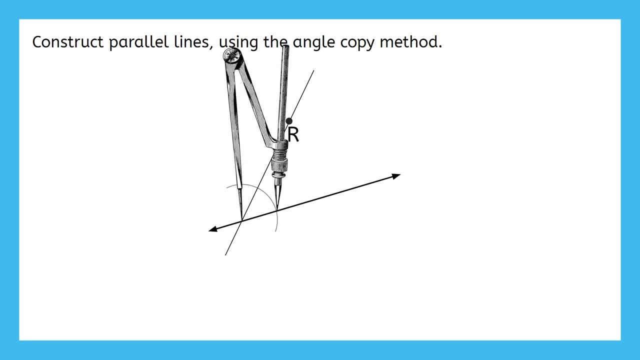 Set a distance on your compass that's not too big and draw an arc where the line and segment intersect. Go up to the new point you made and draw the same arc there too. Then set the distance on your compass where the arc meets up with both your line and segment. 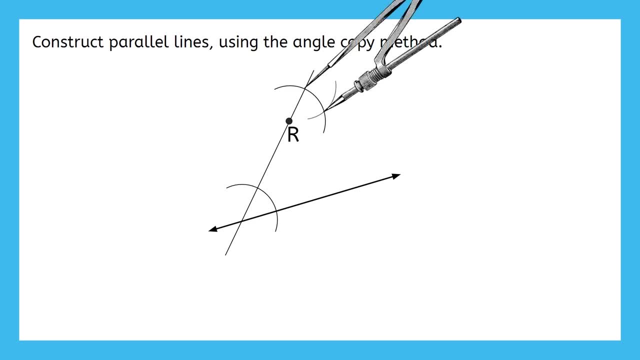 Copy that distance up on your other arc using that same compass. setting Point R in the intersection you just created with your compass is where you'll draw the parallel line. We can make all of our compass marks a little lighter, if we want to, by gently erasing it. 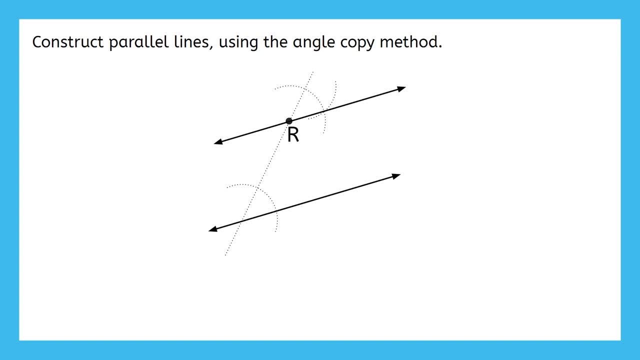 so that it's easier to see the parallel lines. We can mark them as parallel And if we put two points somewhere anywhere on each line, then we can also write a description of what our picture shows. There's some space in your notes template to practice this one more time before we move. 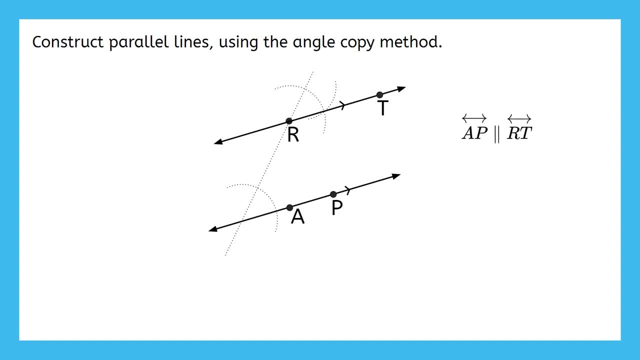 on. so pause the video now and resume when you're ready to learn about a perpendicular construction. Next we are going to go over a method for finding a perpendicular line And actually, more specifically, the perpendicular bisector. We learned what perpendicular means earlier, but 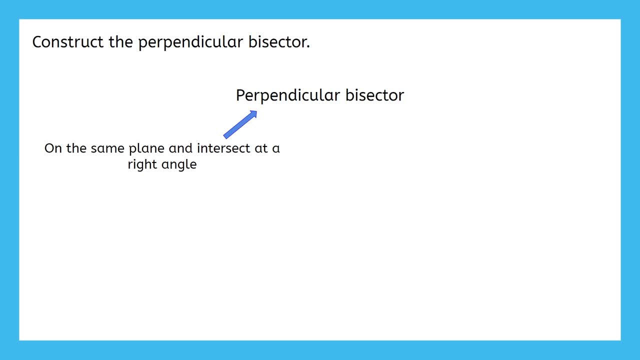 You know what bisector means. Bisect means splitting something into two equal parts. You'll see two other methods in your lesson activity for finding a perpendicular line, but I figured we could look at this more specific perpendicular bisector case together. Remember how a line goes on forever and ever in both directions. 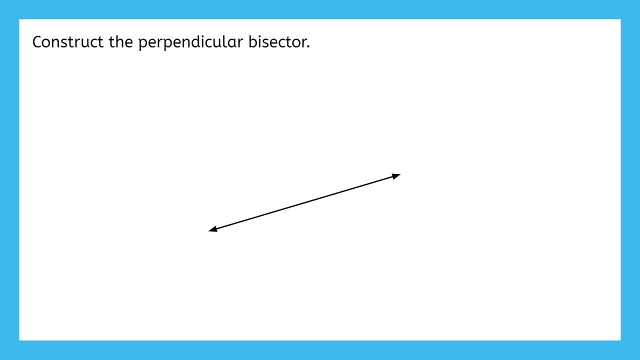 So how do you bisect or split something in half, something that technically doesn't have a bisector? You don't, Which is why we're going to bisect a line segment here instead of a line. Okay, let's get started. 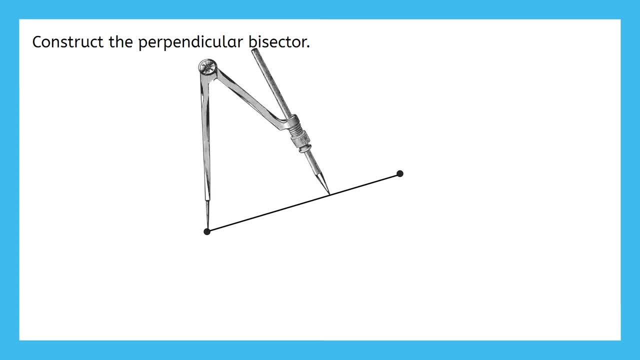 Draw a segment and set your compass so that it's definitely longer than halfway across the segment, but not entirely the way across. Use this setting to draw an arc above and below the segment. Move the compass tip. Move the compass tip to the other end point of the segment and be sure that the setting 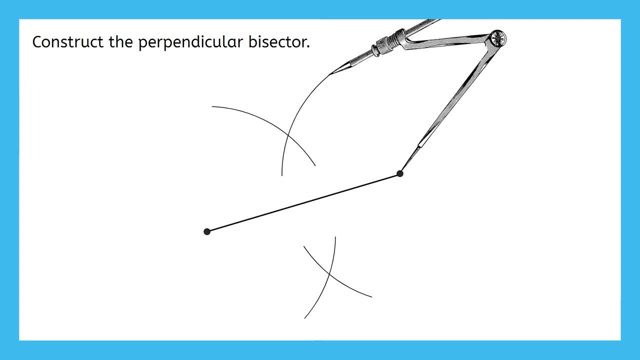 doesn't change. Draw two more arcs, just like what you did before. The two places that the arcs intersect each other are actually the two places we need to draw our new line through. You could just draw a segment here, but I'm going to keep the arrows on the ends of this. 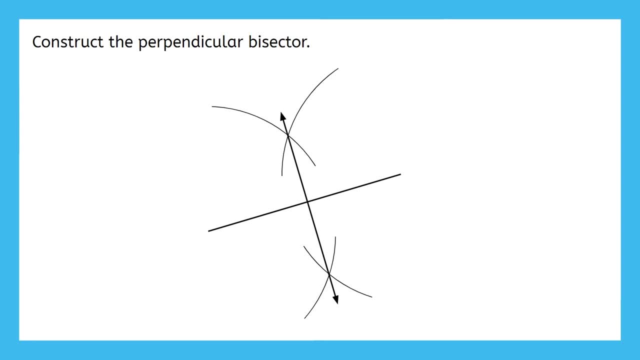 so that it's a line. We weren't told to draw a line here, so we're going to keep the arrows on the ends of this so that it's a line. We weren't told in the directions that we have to write the notation for this, but it's.